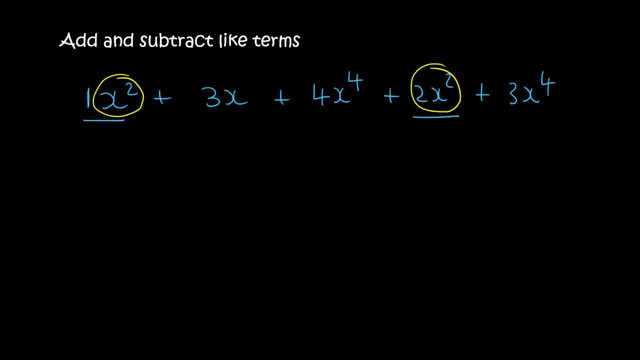 so you've got 1x2 plus 2x2, so that will just give you 3x2.. We're not going to make it 3x4, we're just adding the terms together. Then we've got 3x and there's no other x. 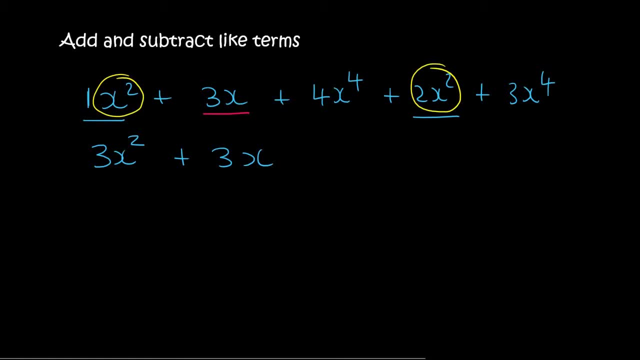 so that's all that you have for the x's. Then you've got 4x4 plus 3x4, so then you'll just have 7x4, and that is the answer. So let's try number one. So for the x squares there's a 3. 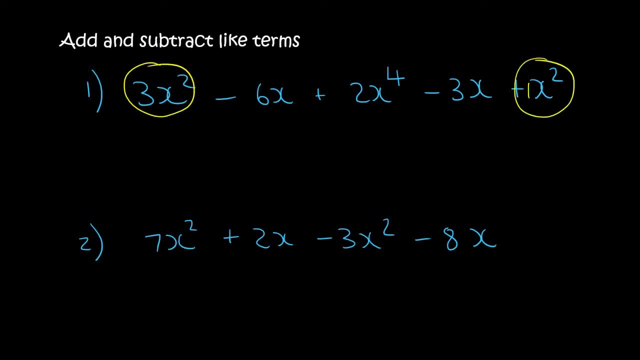 and then over here there's a plus 1, so 3 plus 1 is 4x4.. 4x squared, Then here we've got minus 6x, minus another 3x. So remember if you have minus 6 rand. 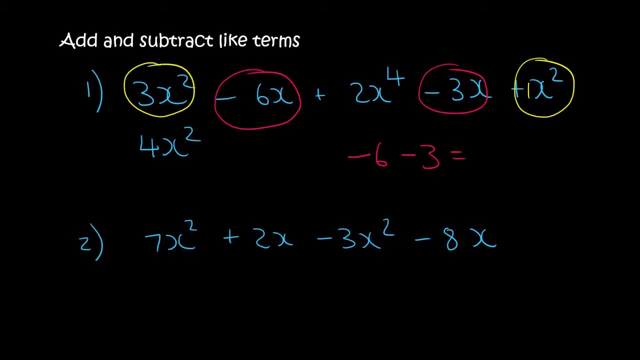 like you owe people 6 rand and then you owe them another 3 rand. now you owe them 9 rand. Oh, but, Kevin, I thought two negatives make a positive. Guys, that's only when you are multiplying or when the negatives are next to each other, like that, But when you are just doing normal. 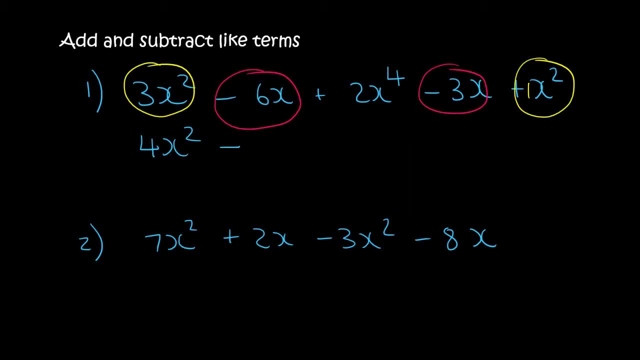 adding and subtracting, you're not going to get a positive, So let's try number one. Then it's not that okay. So that gave us minus 9x, and then the 2x4 is by itself, so that'll just be plus 2x4.. The next one is 7x squared minus 3x squared, so 7 minus 3 is 4.. 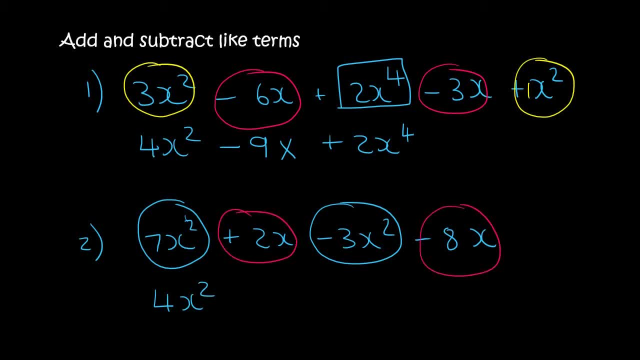 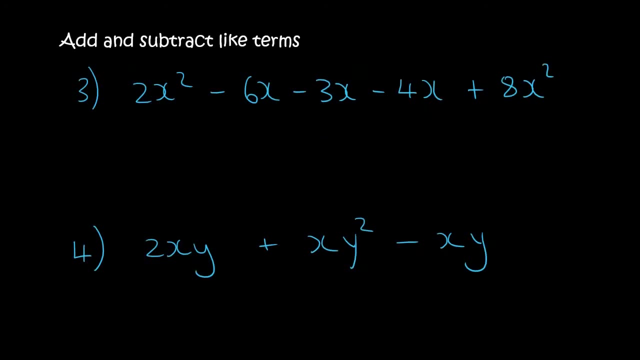 Then you've got positive 2x minus 8.. So imagine you have 2 rand and now all of a sudden you owe people 8 rand. So that's going to leave you with minus 6 and then x. Here's number 3 and number 4.. 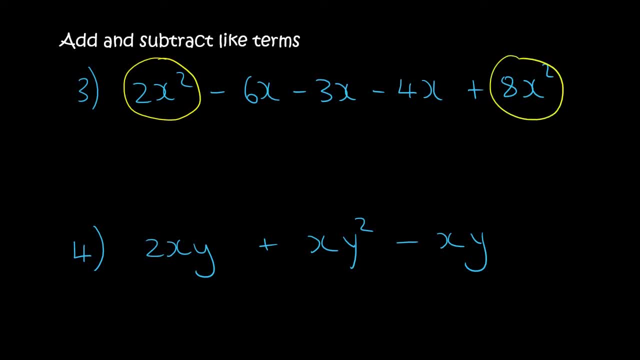 So the x squared? well, there's a 2x squared plus an 8x squared. so 2 plus 8 is 10x squared. Then you've got a minus 6 minus 3 minus 4.. So let's look at that And you can use your calculator. 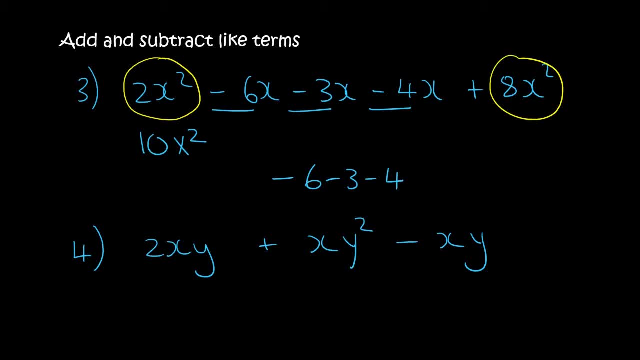 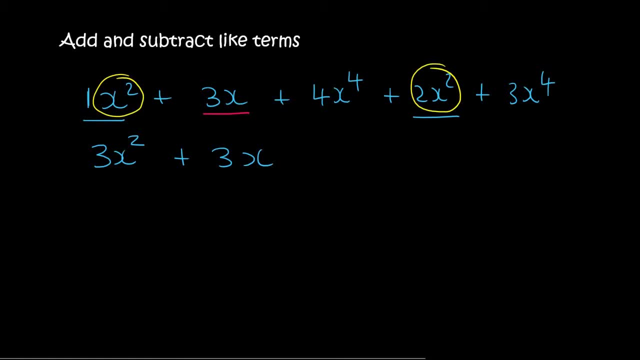 so that's all that you have for the x's. Then you've got 4x4 plus 3x4, so then you'll just have 7x4, and that is the answer. So let's try number one. So for the x squares there's a 3. 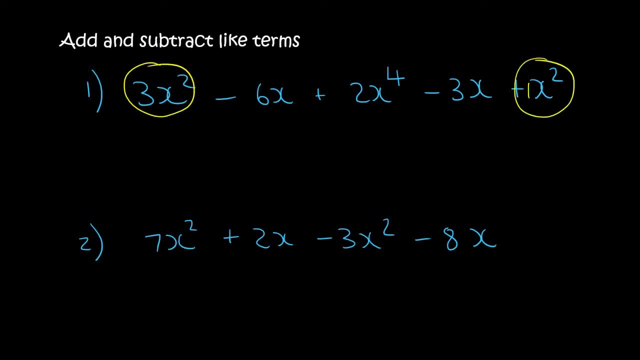 and then over here there's a plus 1, so 3 plus 1 is 4x4.. 4x squared, Then here we've got minus 6x, minus another 3x. So remember if you have minus 6 rand. 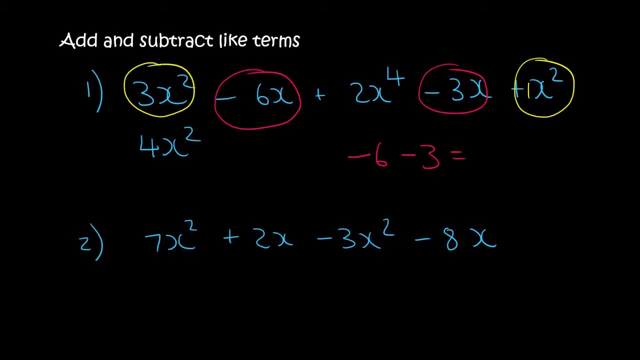 like you owe people 6 rand and then you owe them another 3 rand. now you owe them 9 rand. Oh, but, Kevin, I thought two negatives make a positive. Guys, that's only when you are multiplying or when the negatives are next to each other, like that, But when you are just doing normal. 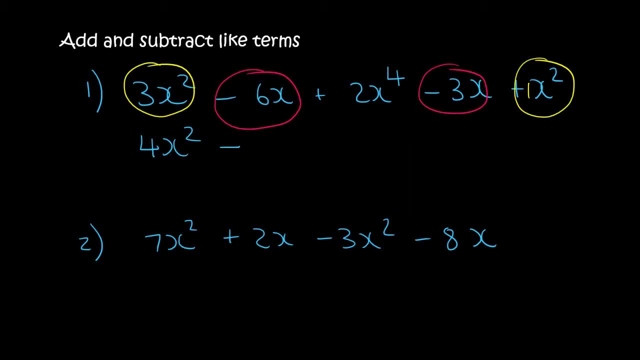 adding and subtracting, you're going to get a negative. So you're going to get a negative, Then it's not that okay. So that gave us minus 9x and then the 2x4 is by itself, so that'll just be plus 2x4.. The next one is 7x squared minus 3x squared, so 7 minus 3 is 4.. 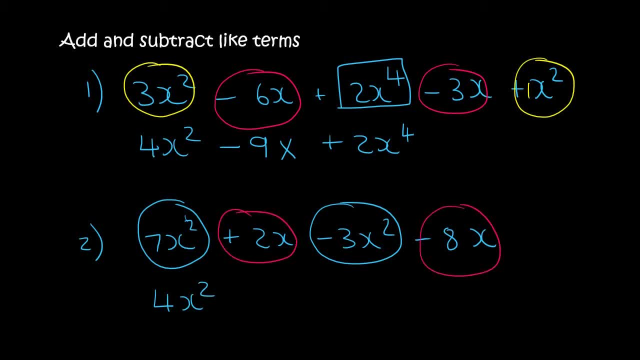 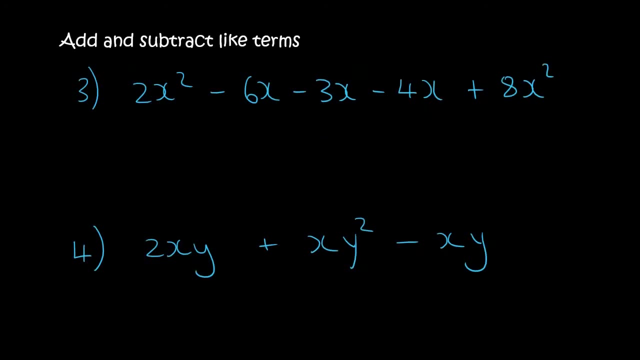 Then you've got positive 2x minus 8.. So imagine you have 2 rand and now all of a sudden you owe people 8 rand. So that's going to leave you with minus 6 and then x. Here's number 3 and number 4.. 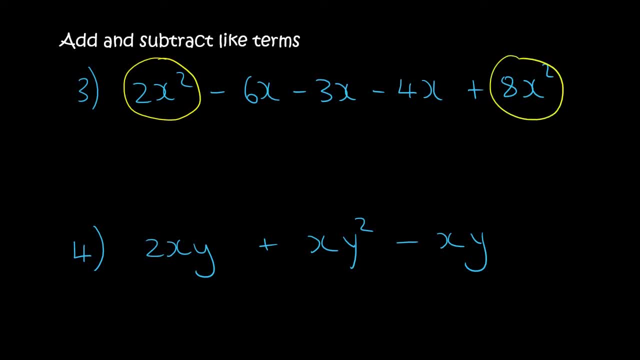 So the x squared? well, there's a 2x squared plus an 8x squared. so 2 plus 8 is 10x squared. Then you've got a minus 6 minus 3 minus 4.. So let's look at that And you can use your calculator. 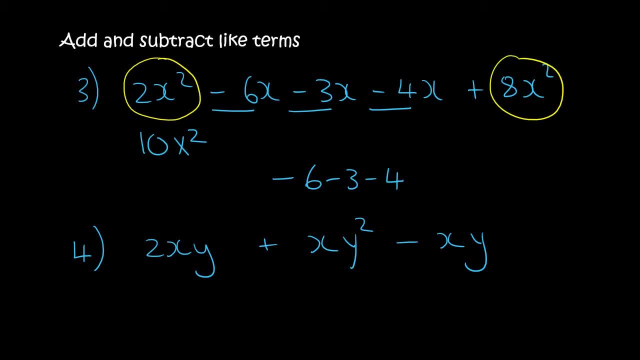 I tell my students to just use a calculator. It just makes life easier. So you could type that in the calculator. but if you want to do it old school, then minus 6, so you owe people 6 rand. Then you owe another 3 rand. So now you owe a total of 9 rand. Then you owe another 4 rand. 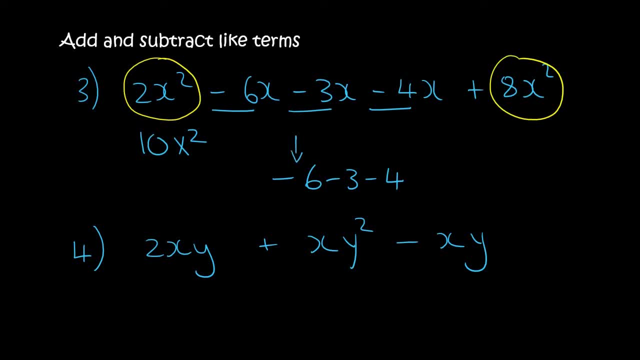 school, then minus 6, so you owe people 6 rand, Then you owe another 3 rand, So now you owe a total of 9 rand, Then you owe another 4 rand, So you owe a total of 13 rand, And so that's going to be. 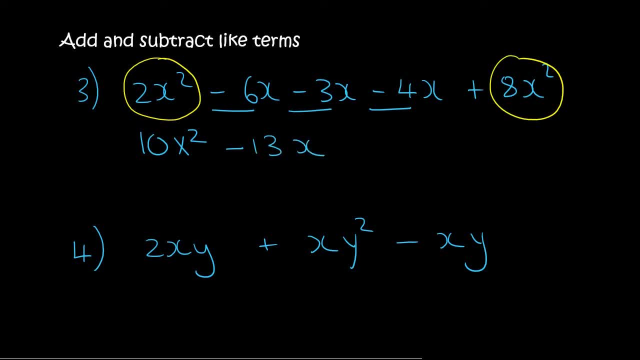 minus 13x. This one over here. students get a little confused. xy is not the same as xy to the power of 2. It is the same. It is the same as this one because that's xy. So we have 2xy minus 1xy. Remember the number in the? 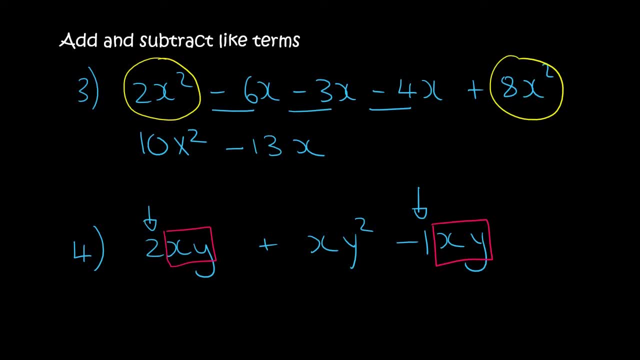 front is a 1 if there's nothing there. So 2 minus 1 is just 1.. So you can say 1xy, or you can just say xy, It doesn't matter. And then this one is just by itself, And there we have it. Okay, so number. 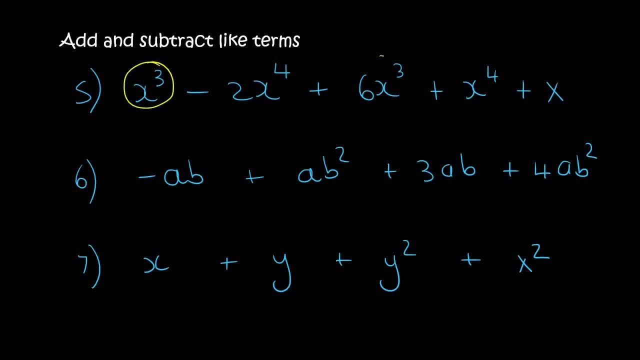 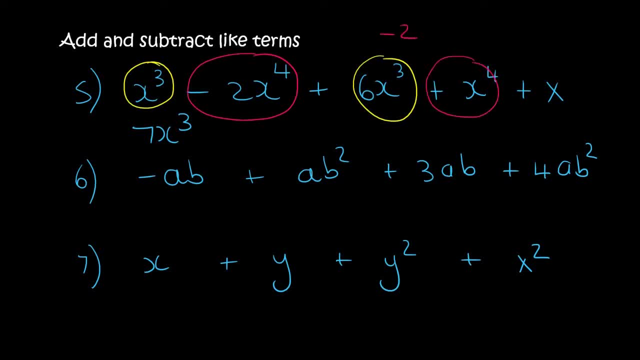 2x4 plus x4.. So it's minus 2 plus 1.. So if you owe someone 2 rand and then someone gives you 1 rand, well then you only owe a total of 1 rand. So that'll be minus 1.. But remember, use the 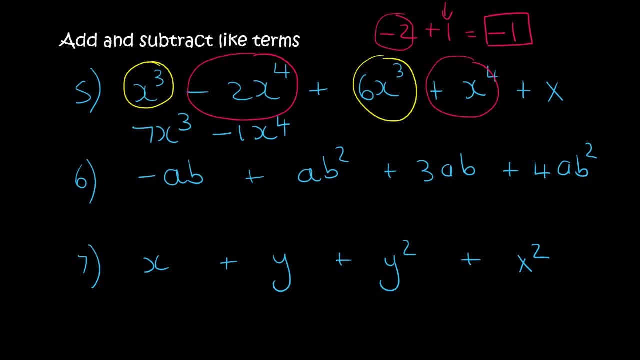 calculator. It's absolutely fine. It's just going to make your life so much easier. And then all that we have left is this little guy, And so that's just going to be plus x. Moving on to the next one. So here we've got a minus 2 plus x4. So that's minus 2 plus x4. So that's minus 2 plus. 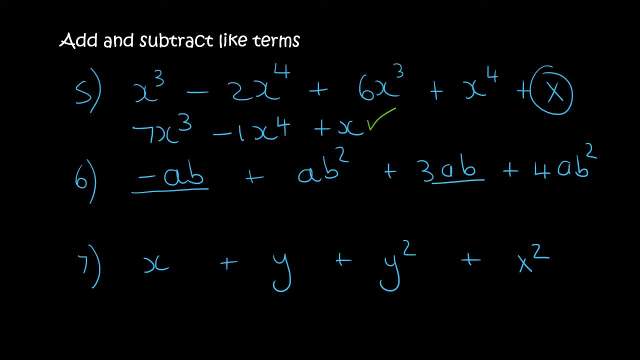 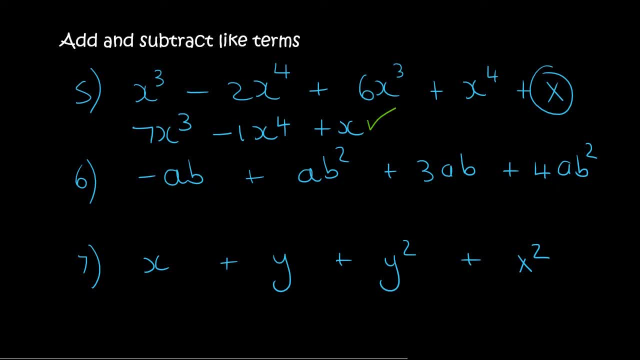 Although they have a's and b's, their exponents are different. So we've got minus 1 plus 3.. So you use your calculator: Minus 1 plus 3, and that'll give you 2. So that'll just be 2 a b. 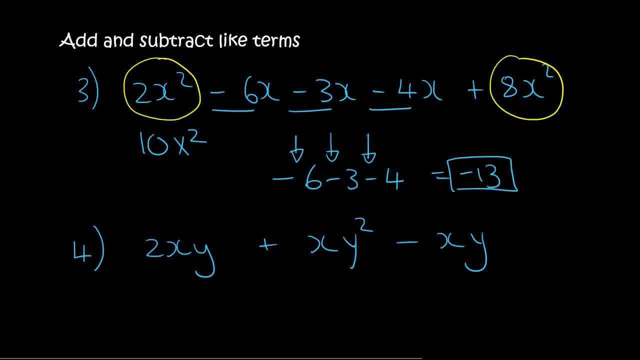 So you owe a total of 13 rand And so that's going to be minus 13x. This one over here students get a little confused. xy is not the same as xy to the power of 2. It is. It is the same as this one because that's xy. So we have 2xy minus 1xy. Remember the number in the? 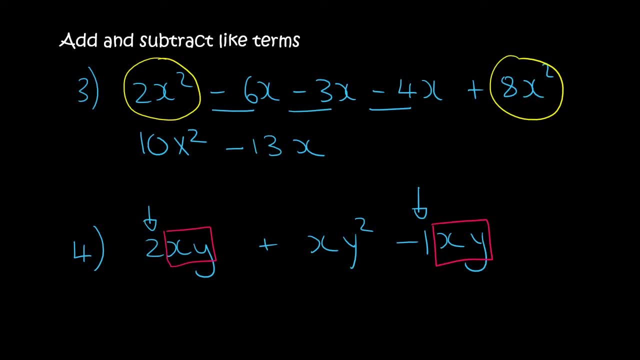 front is a 1 if there's nothing there. So 2 minus 1 is just 1.. So you can say 1xy, or you can just say xy, It doesn't matter. And then this one is just by itself, And there we have it. Okay, so number. 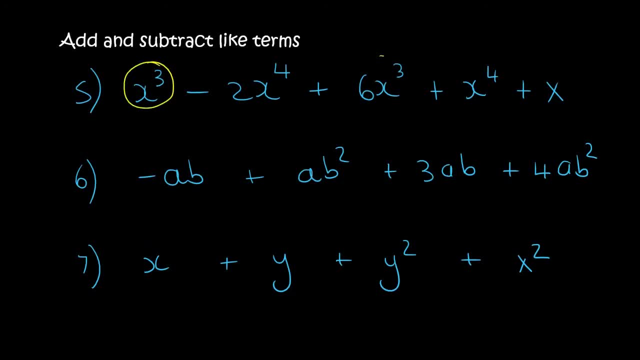 5, we look for the like terms. There's an x3 plus 6x3. So that's 1 plus 6, which is 7x3. Then you've got minus 2x4 plus x4. So it's minus 2 plus 1.. So if you owe someone 2 rand and then someone. 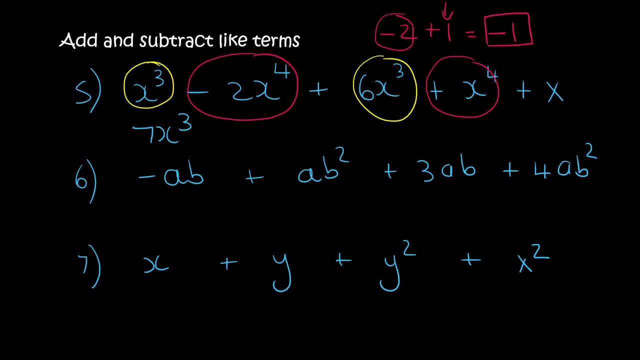 gives you 1 rand. well then, you only owe a total of 1 rand, So that'll be minus 1.. But remember, use the calculator. It's absolutely fine. It's just going to make your life so much easier. 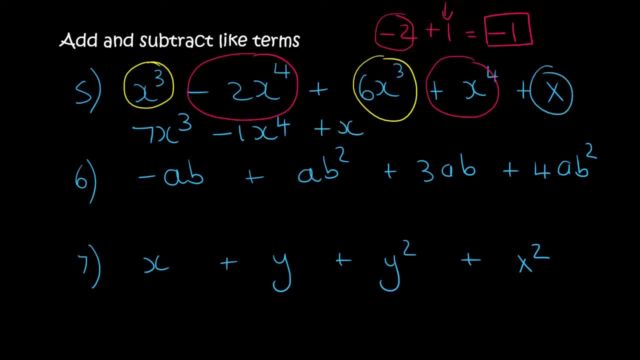 And then all that we have left is this little guy, And so that's just going to be plus x, Moving on to the next one. So here we've got a minus ab, And then we've got another ab over here. It's not the same as ab. 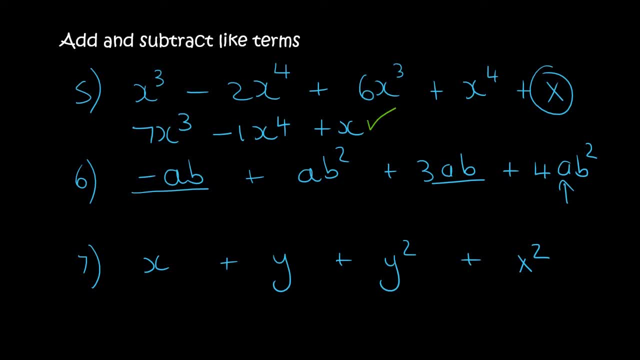 squared and ab squared, They are different. Although they have a's and b's, their exponents are different. So we've got minus 1 plus 3.. So you use your calculator: minus 1 plus 3, and that'll. 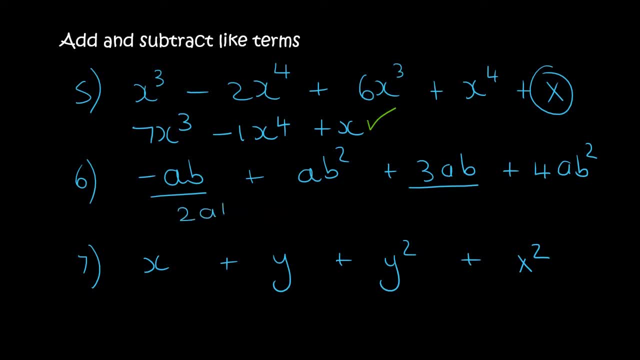 give you 2. So that'll just be 2ab plus ab squared plus 4ab squared, So it's 1 plus 4, which is 5. It'll be plus 5ab squared. With this one, nothing is the same, That is not the same as that, And so 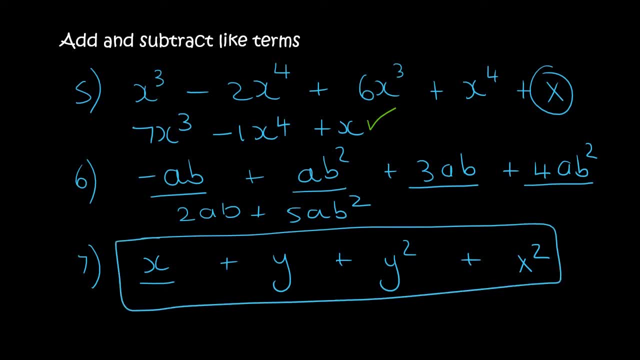 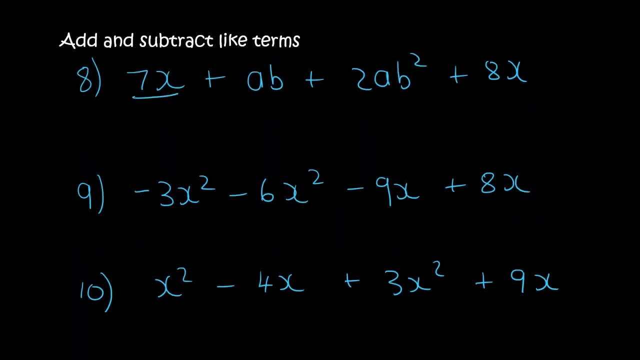 this is the answer. It's a trick question. There's nothing you can do here. You cannot add and subtract them if they're not the same Number 8.. So we've got an x there and an x there, So 7 plus. 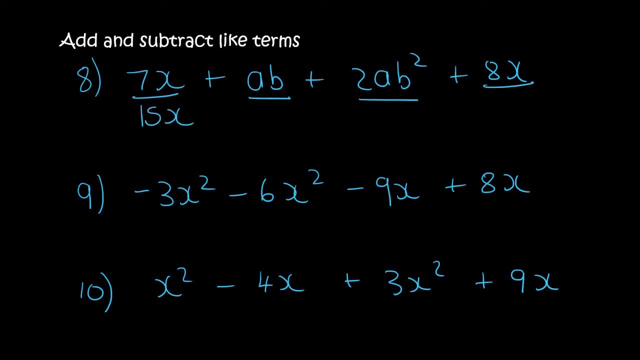 8 is just 15.. So that's 15x. Then these two are different, So you can't put them together, So they will stay separate like that. Then this one minus 3 minus 6. So you can type it in on the calculator and that'll just be minus. 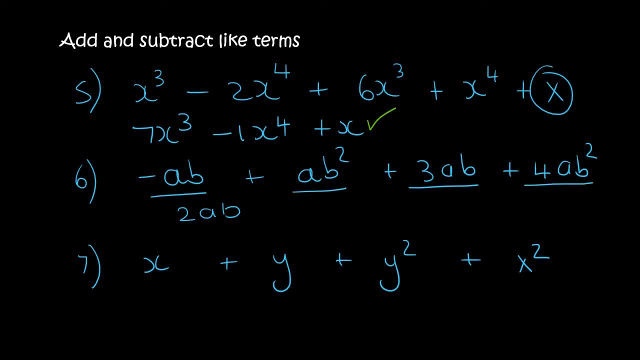 plus a b squared, plus 4 a b squared, So it's 1 plus 4,, which is 5.. So it'll be plus 5 a b squared. With this one, nothing is the same, That is not the same as that, And so this is the. 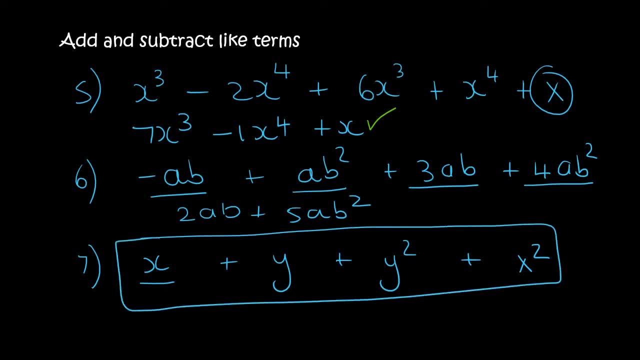 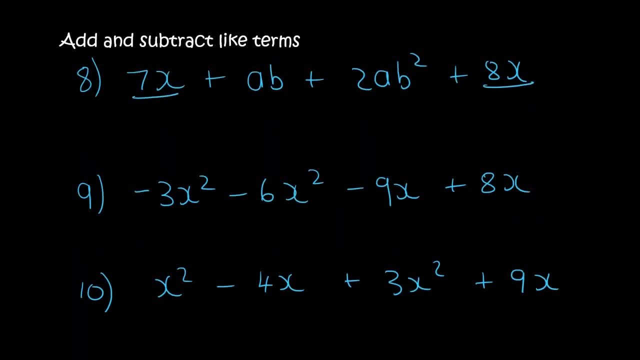 answer. It's a trick question. There's nothing you can do here. You cannot add and subtract them if they're not the same Number 8.. So we've got an x there and an x there. So 7 plus 8 is just 15.. 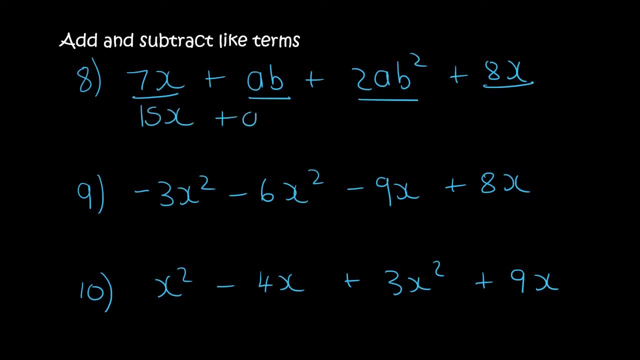 So that's 15x. Then these two are different, So you can't put them together, So they will stay separate like that. Then this one minus 3, minus 6. So you can type it in on the calculator and that'll just be minus 9x squared. 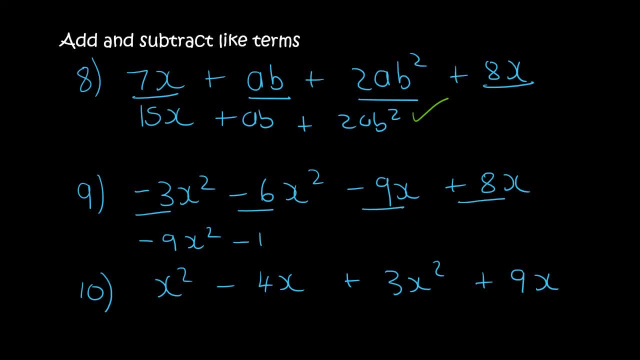 And then these two are the same, So it'll be minus 9 plus 8, which is minus 1x all. coming from the calculator, This one will be x squared plus 3x squared, So that's 1 plus 3,. 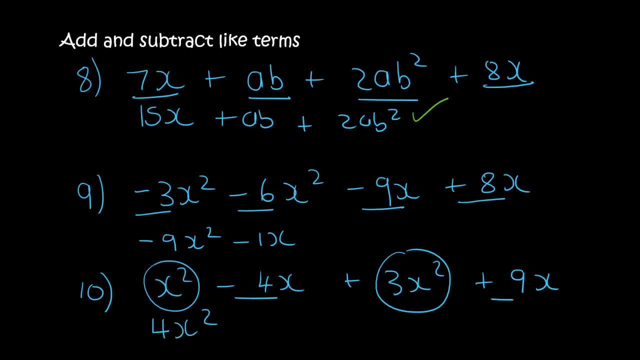 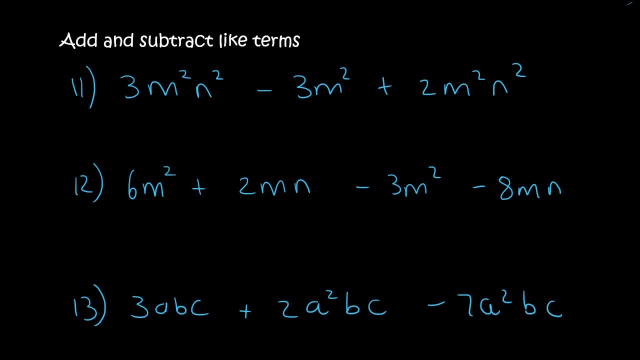 which is 4.. And then minus 4 plus 9.. Just use the calculator: Minus 4 plus 9 is 5.. And there we have it, So number 11, we can see that this is the same as that. So we can put them together. So that's 3 plus 2,. 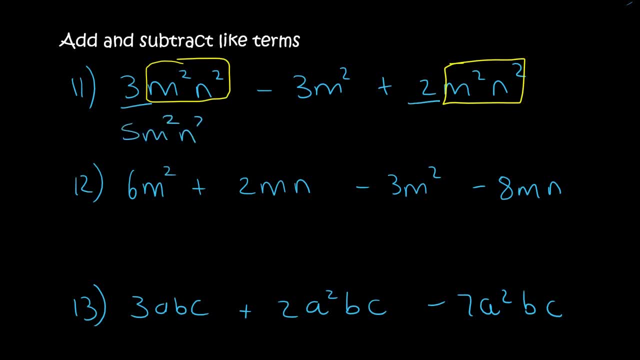 which is 5.. But then it doesn't become a 4. You leave it as it is, And then this part is just hanging by itself. So like that, Now we've got an m squared here and an m squared here, So that's 6. 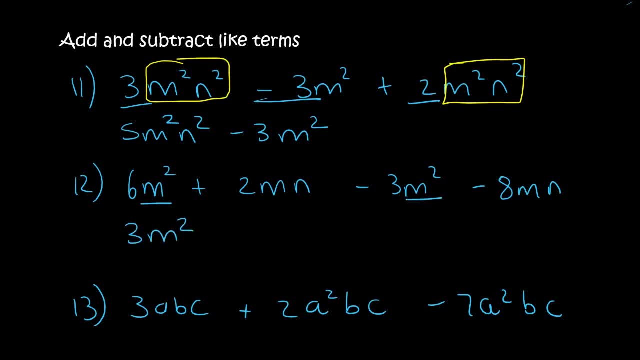 minus 3, which is 3.. Then you've got a 2 minus 8.. So you just use the calculator if it gets a bit complicated and you'll just be left with minus 8.. So that's 2 minus 8.. So you just use the calculator. 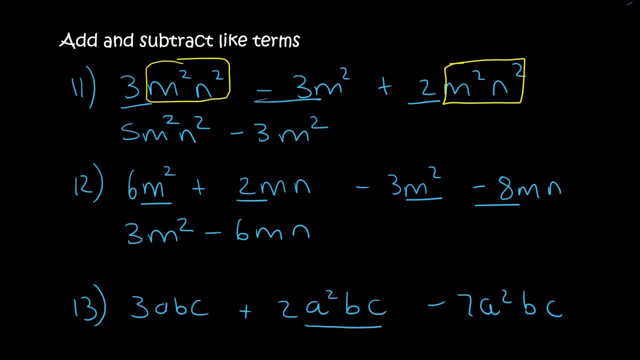 minus 6.. Then these two are the same, So that becomes well, let's do this part first. So that's just by itself. So it's 3abc Now, 2 minus 7.. Just use the calculator, That'll give you minus 5a. 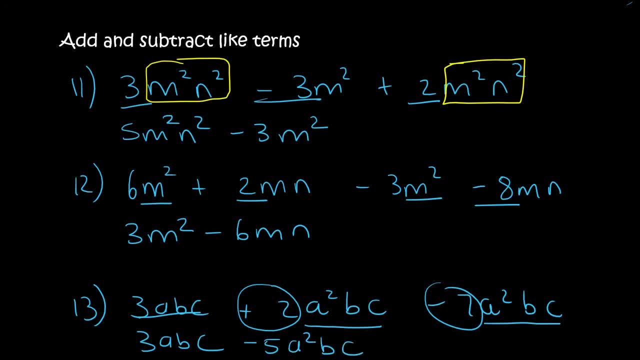 squared b and c. So, guys, in this lesson we looked at how to add and subtract like terms.